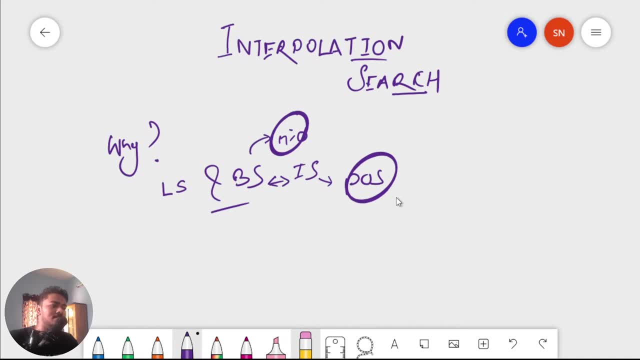 it uses to calculate that where does this thing may exist, and it directly goes to that area or the or different areas, instead of just searching in the middle. so that makes a little bit of optimization over binary search and we're gonna see in this video what is that formula and 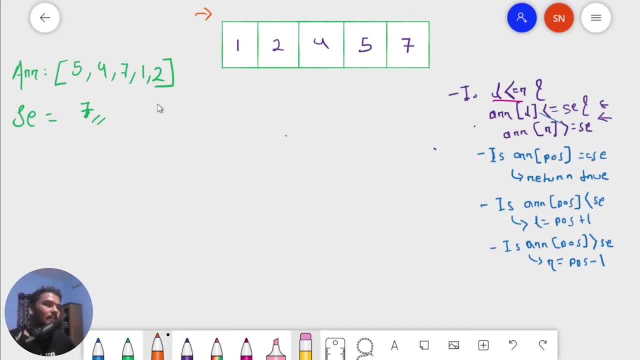 how does this work? okay, so let's assume we have the array five, four, seven, one, two and we have to search seven. right, we have to search seven. so, as you can see here, i've already sorted the array. in short, if i say why we sort, is that this sort sorting arranges the elements from a lesser to a. 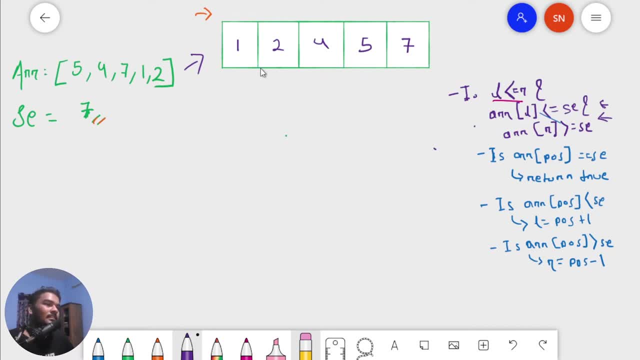 greater side. so, for example, you know now where our element lies. if it is less, it will be obviously in the left side. if it is greater, it will be obviously on the greater side. now, if you just see this checks right here, you will just totally find that they are equal to what binary search? 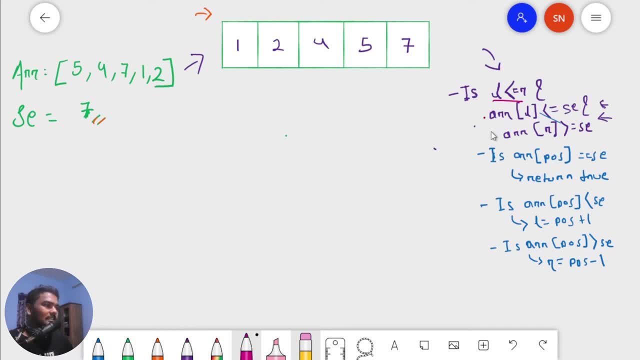 steps are. except just these two checks, everything is equal to binary search, um, so we will go through everything, so don't worry about that. so let's just get started solving this um, going through how this algorithm works. okay, so, exactly like binary search. we just need to play around with three variables and everything will be. 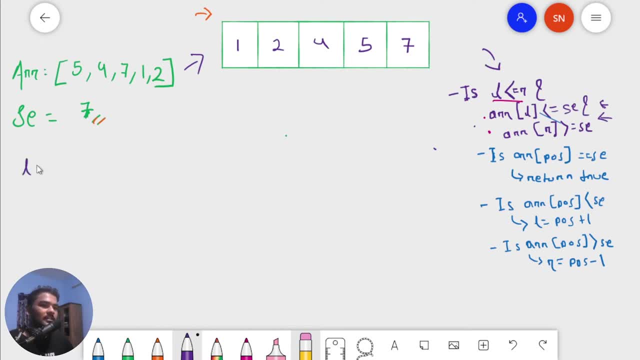 done so these three variables are: left, the left most position, the r, which is the right most position, and here where we had the middle element, actually, uh, in case of the binary search, where its formula was l plus r by two, but instead here in interpolation search, we have to just find a. 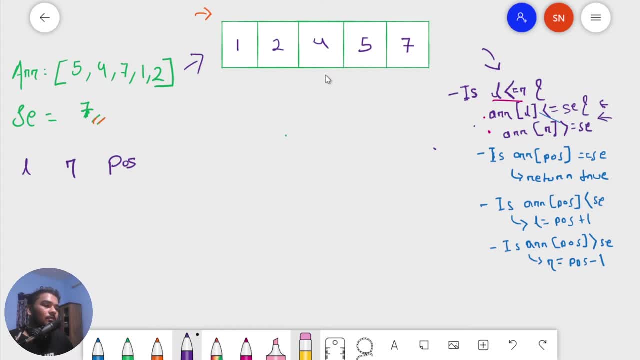 position, not just middle. so this position can be anywhere and it has also a formula. and this is how the formula is actually. it just looks long. so this is how its formula looks like. so here i'm writing um. so this is goes something like this: so l left most position plus right most. 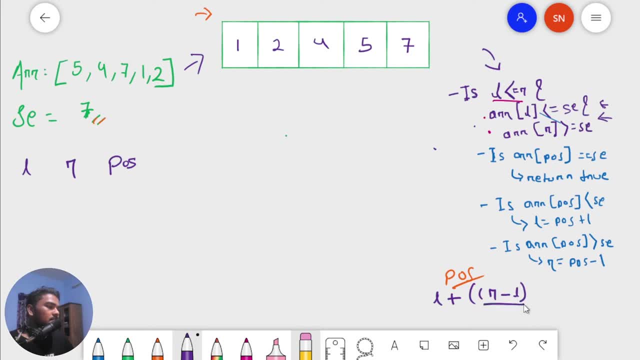 position minus left: most position divided by the element in the right. most position minus the element in the left: most position into the search element minus the element in the left: most position right. so this is exactly so. this is the formula of position. so now you must be asking: well, why do we need this position right? so this position is: 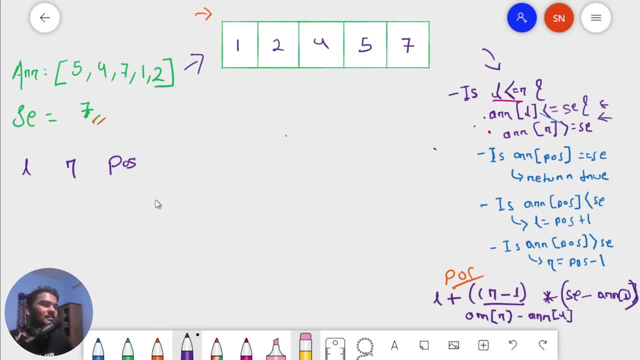 everything that makes one that optimizes interpolation search over binary search. because this position that you will get is according to where is the most probability that the number would lie. because, for example, if you are searching for one in this array, it makes more sense to just see where, in which region, the number may lie, and just go to that region directly instead of just 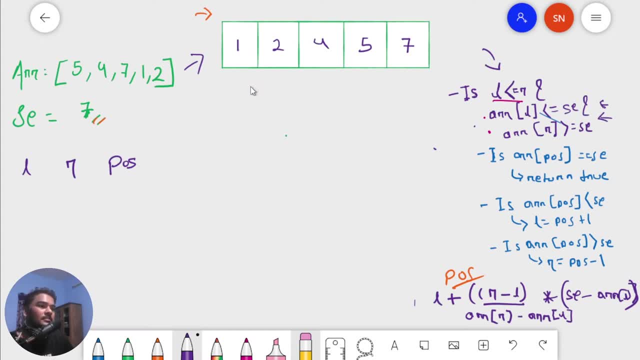 going through middle and middle and middle, right, as we do in binary search. so that's how interpolation search actually optimizes over binary search. and you will see this because on this problem i will be also doing binary search and we will compare how many steps does it take, right? so let's get 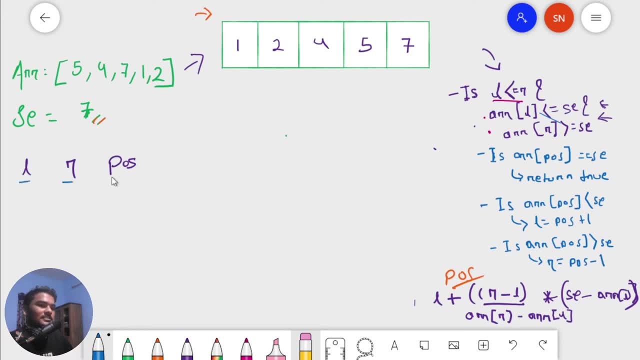 started now. so let us maintain just this table to see how we are actually going. okay, so first, as we know, at our left most position- we are here so because we are starting- and then the rightmost position: 0, 1, 2, 3, 4. so this is where. 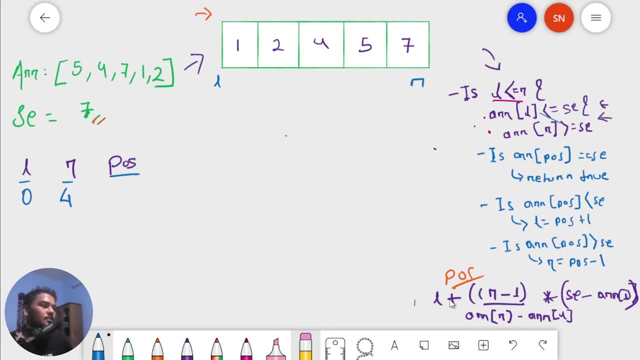 we are, and the position. let's put the formula, let's put this formula right, um so l is 0 plus r minus l, 4 minus 0 is 4. then by the position, the element in the rightmost position, 7 minus the element in the leftmost position, that is 1. so 7 minus 1 is 6, and 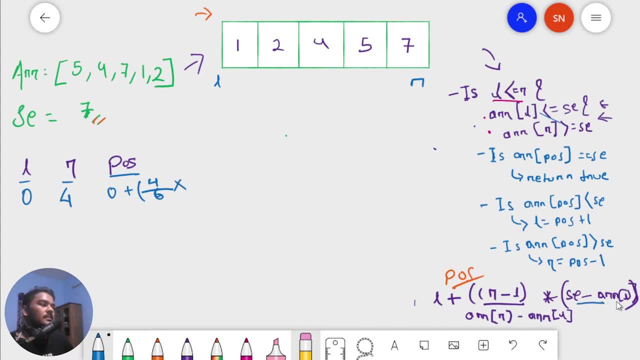 into search element minus the element in the left leftmost position. so search element is 7 and the element in the leftmost position is 1 right, so that is 6. so if we just cut, cut and the position we get is 4 right. so this is how the table is. as we have got these three variables, we go through. 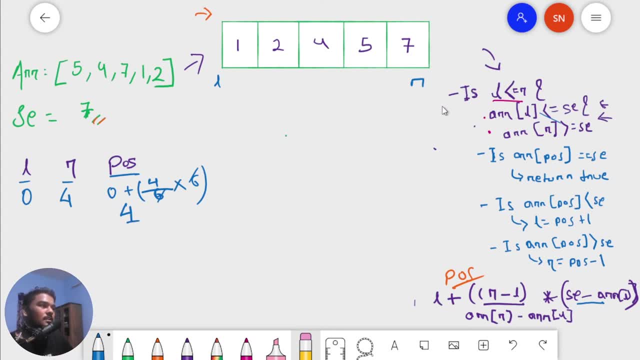 our checks right. so this is the bigger check, this purple one, and if this validates, only then we go to the search element and if we just return false, that we have not got the like the thing we are searching for is not there. so let's get into it. is l less than equal to r? yes, 0 is less than equal to. 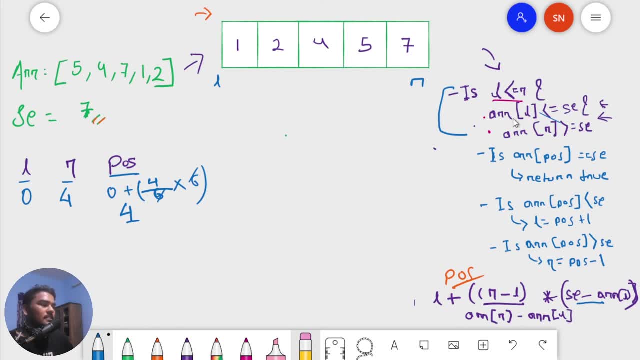 r. that's fine. and and is the element in the leftmost position, less than the search element? yes, 1 is less than 7. um. and is the element in the rightmost position, 7 is less greater. is greater than equal to the search element? yes, it is. 7 is greater than equal to 7. so 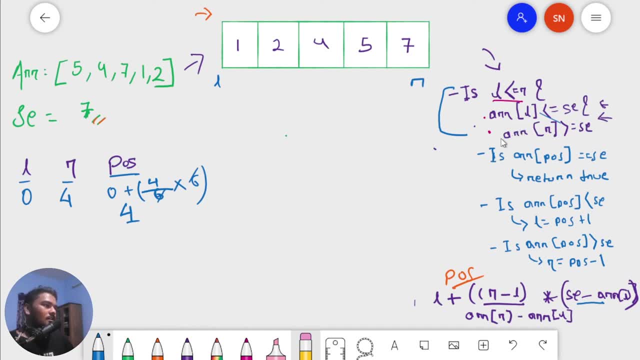 everything passes right and then we get to the these smaller checks. so is the element at the position, at the fourth position, equal to the search element? yes, it is, because the at fourth position is 7 and we are also searching for 7.. I mean, it's that fast, right? it just got us the answer. 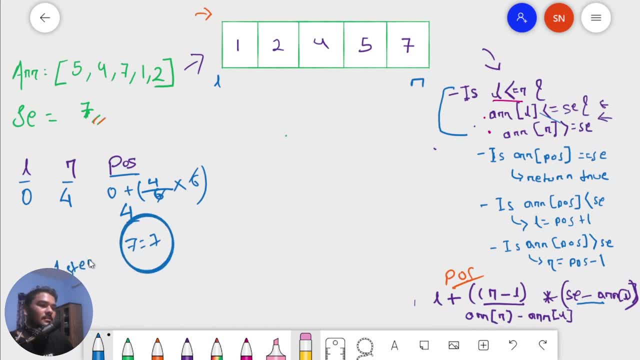 in one step, right. so we just took one step, right, and we have the answer now. now let's just do this thing with the binary search. okay, let's do just same thing with binary search and just assume that these two points now don't exist, because in binary search these, we don't consider these two points and just assume that these. 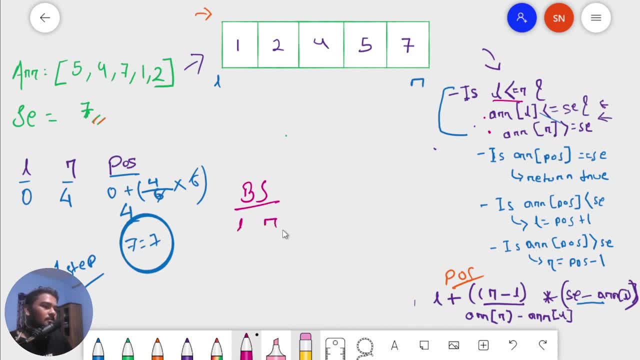 positions at the mid. okay, we are talking about. so let us make this table l, r and mid, like we do in binary search, and we will start with zero four, because we are at the first now, and then the mid. how do you calculate? made in binary search, l plus r by two, so four by two is two right now. so 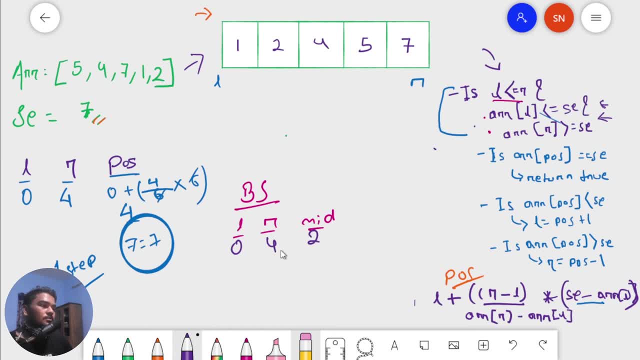 both of the checks. so is left less than equal to r. yes, zero is less than equal to four. great, so now we have passed this test. now let's go to the smaller, smaller checks. is the element in the middle equal to the search element? so in the? so here we are now right. and the four is four equal. 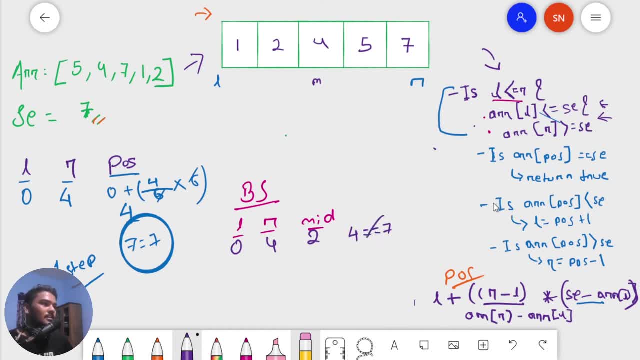 to equal to seven? no, it's not. so now let's get to the second condition. so is the element in the middle less than the search element? yes, it is, because four is obviously less than seven, right? so now let me just go a little bit deep into it and let me tell you how, why we sort, and you'll. 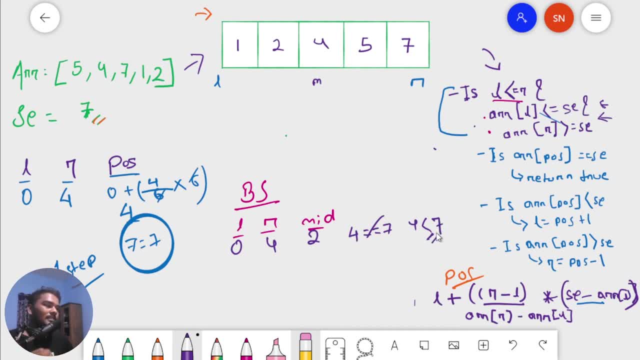 understand now. so as we have sorted this. so how this helps us now is that the seven, as the seven is greater than this middle element four, so obviously as it's, it is sorted, and seven is greater than four, obviously seven must lie on the right side of four, right, because it is sorted. so 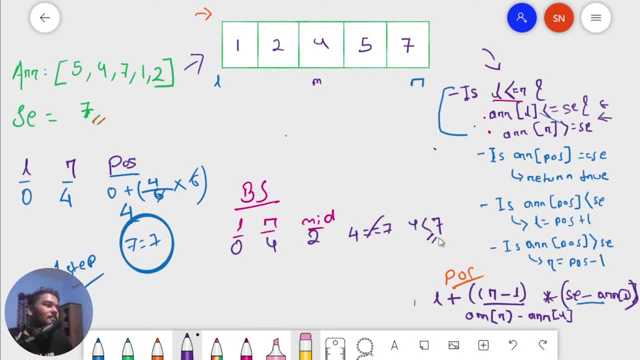 it could be according to a particular position, right. so, as it is in the right, so it is somewhere here, right? this is what we know now from the algorithms, from the algorithm. so it is somewhere here, so we don't need to actually consider this part anymore. so what we do now is that just bring. 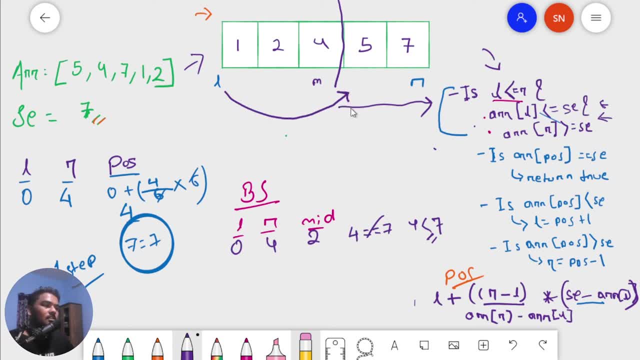 this thing here. this is basically binary search logic, right? and how do we bring it here? so that's why we do: here l is equal to position plus one, or here, in this case, mid plus one, right? so l will now come here, so l will be made plus one. now it is three, so now we will be considering just this area. 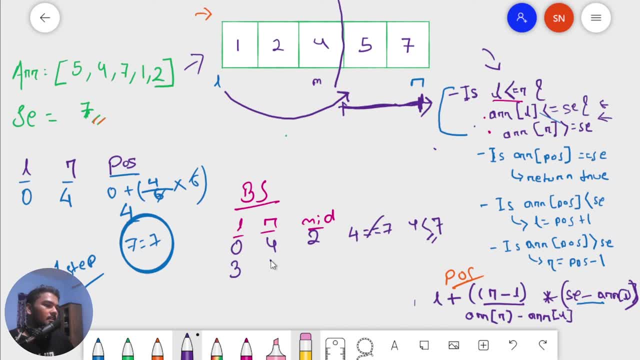 right, just this area. so r will remain same four. so four plus three, seven by two is three. so now let's check. is l less than equal to r? yes, three is less than equal to four. so is now the element in the middle position equal to the search element? no, because now we are here, right, l is here, our. 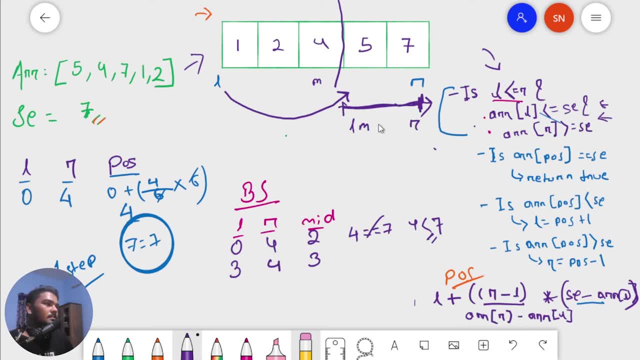 mid is also here, so the element in the middle position is five. five is obviously not equal to seven, so let's go to the next check. so is the element less than search? yes it is. five is less than seven. okay, so that tells us that the thing we are searching for, that set that seven, is obviously on the right side of our 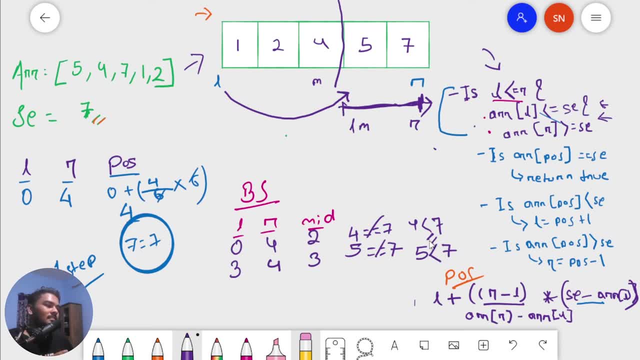 this middle element right, because it is greater than this middle element right, so it is somewhere now here. so now we make our l go here now. so how we do that again, we do l mid plus one, right, and so now the l will be four, because three plus one is four, then four, and if you just 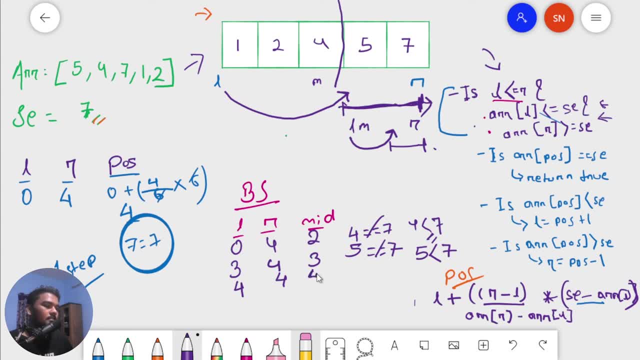 uh, find the mid. now it will be eight plus eight by two, that is four. right now. is l less than equal to r? yes, four is less than equal to four. and is the middle position? is the element in the middle now equal to the search? yes, it is, because we are at four now. everything, lrm, everything is here, so 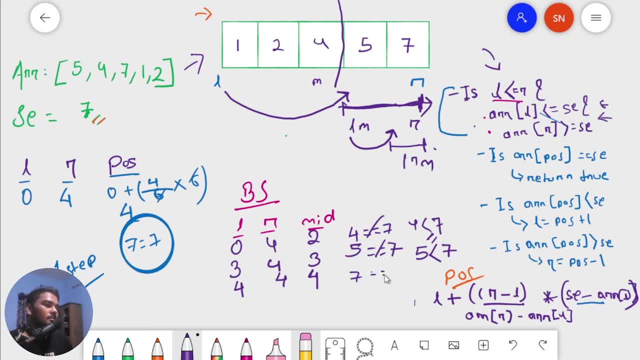 seven is at the fourth position and the element we are searching for is also seven. so we have found it. so how many steps did it actually take? so we took one, two, three. so binary search took three steps right, and if you just compare it to interpolation search, it took one step right. so 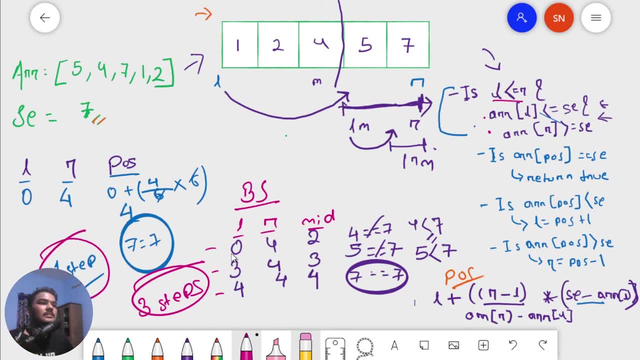 that's how interpolation search is optimizing binary search. it is not just going through and calculating just the middle element, these middle elements. instead, it is calculating the most probable area where the, where the element we are searching for could be according to its size, right? so, as seven was a really big thing, it was- it should be at the uh, at the highest end, right. so? 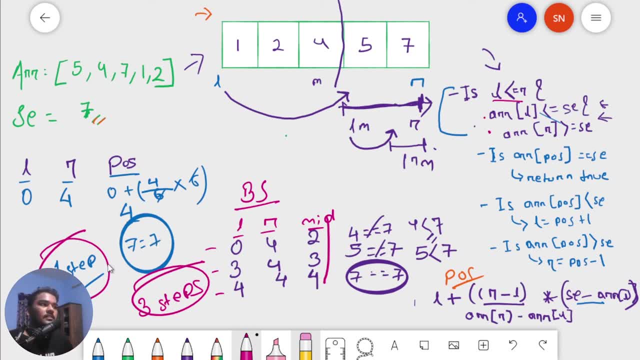 it just took us to the highest end and guess what. we have found this right. so that's how interpolation search works. so i hope you understood the working of interpolation search. if any doubt, just mention it in the comments, i'll be obviously you replying. so now let me show you the code. that will just clear everything out. okay, so this is. 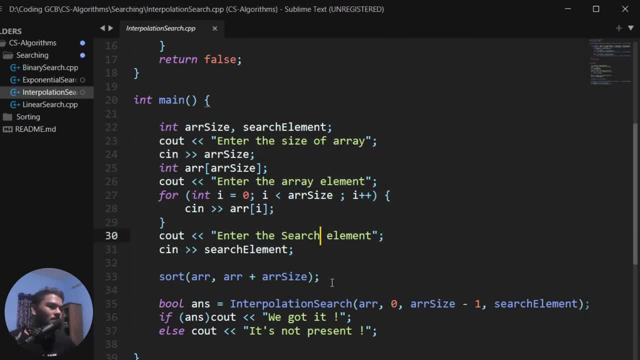 a code. just ignore this part, because here i'm just taking input and stuff. so here the real thing begins. we have sorted the array as we told you we need to sort to you know know, the positions actually according to the size, and here we then call the interpolation search function and pass. 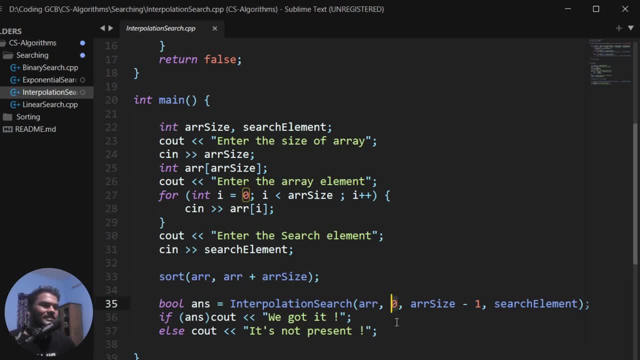 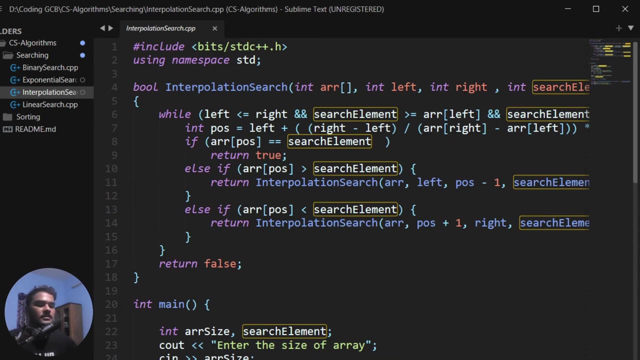 the array into it: the leftmost position, which is, which is at the starting zero, then the rightmost position, which is the length of the array, basically minus one, because you know it's um zeroth index. then we're just passing the search element and this thing, and this is actually what the function looks like: interpolation, search- and if you just, uh see, 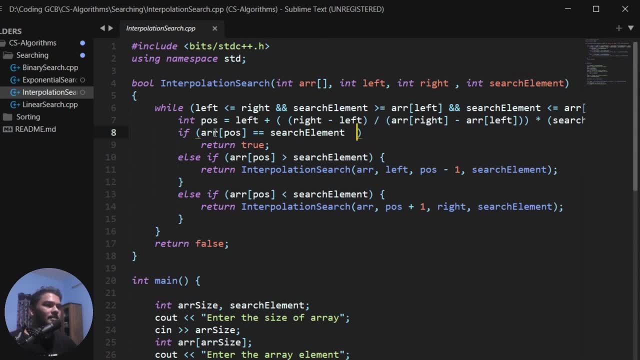 you will and compare the thing i told you, you'll find it's exactly that. uh, here is the condition, the bigger condition which it needs to pass to go through these three, uh, smaller conditions, right. so first we check: is left is less than equal to right? then we just check. 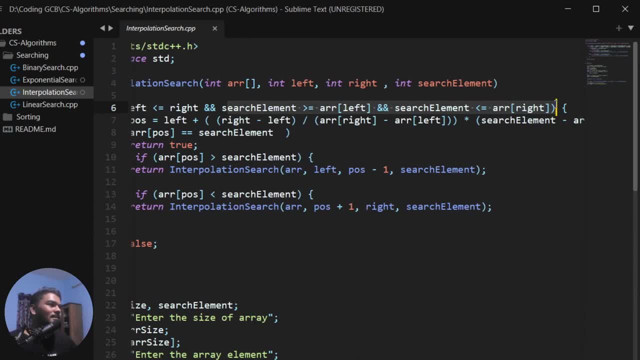 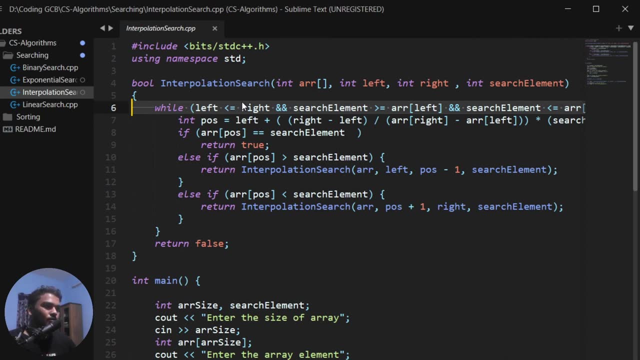 and these two things, this, these line, just say that is this search element between the element at the left and the element at the right, and if we pass through it, obviously, then the thing we are searching for is in the array. so we go to next steps. here we find the position with the. this is: 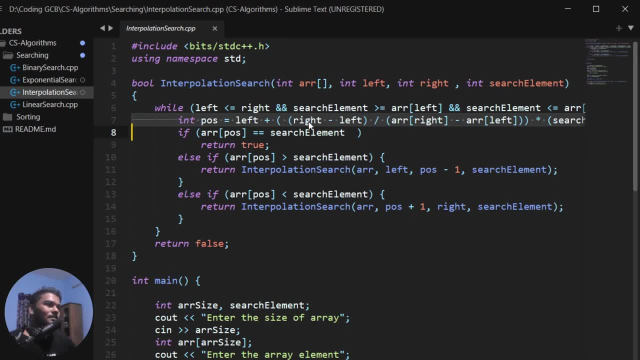 the formula we talked about, of the position, and obviously you will find the code in the description and obviously, and also the github repository where i'm maintaining all these algorithms so that you can, you know, fork it or you know, use it. so now we just that we have the position and stuff, we just check through these three things, right and whatever.